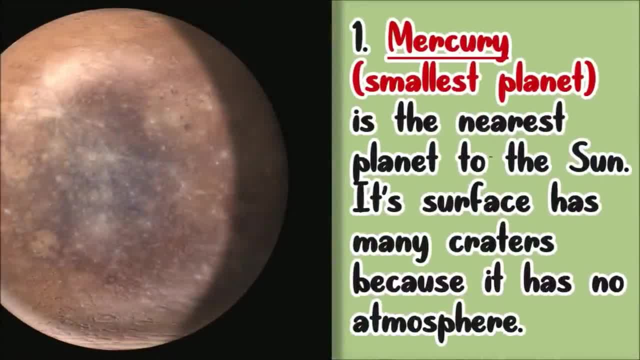 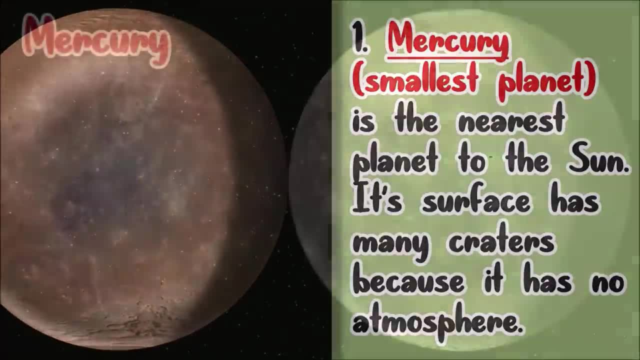 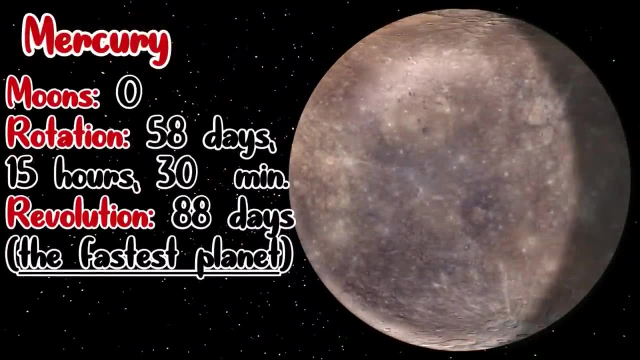 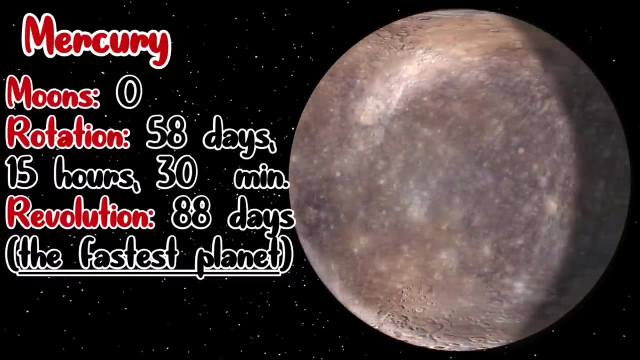 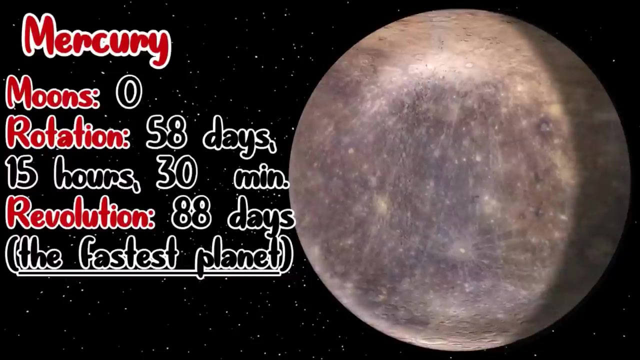 Mercury is the nearest planet to the sun. Its surface has many craters because it has no atmosphere. Mercury has no moons. One rotation of Mercury is equivalent to 58 days, 15 hours and 30 minutes. However, it requires 88 days in one revolution on the sun. That is why it is considered as the fastest. 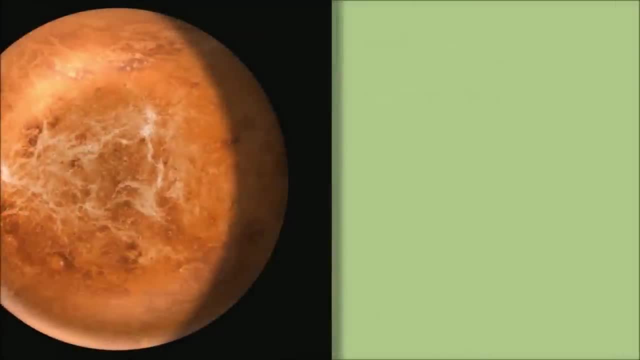 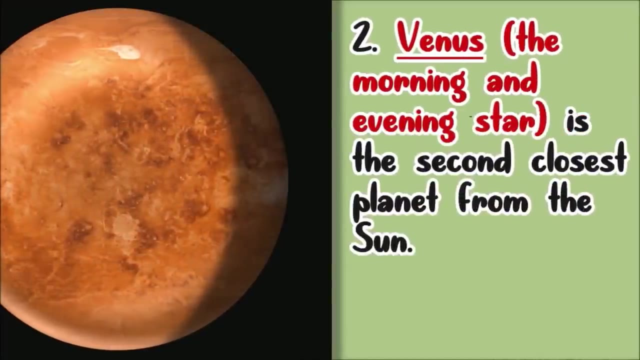 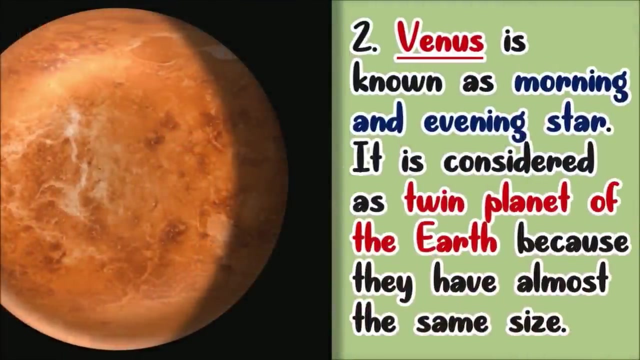 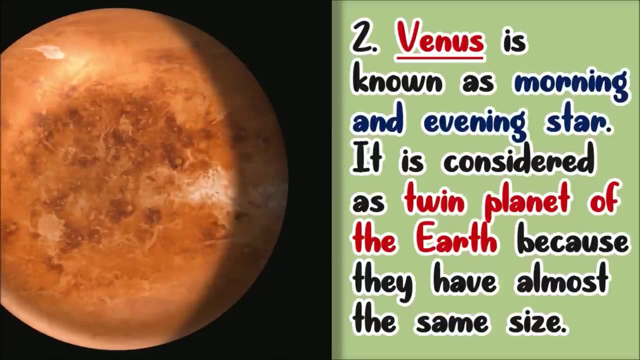 planet Venus. It is the second planet from the sun, Aside from the sun Venus. Venus is the brightest object in the sky. Venus is commonly referred to as the morning and evening star. It is also considered as the twin planet of the earth. 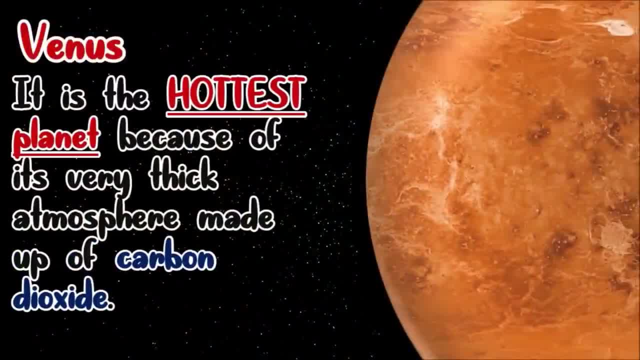 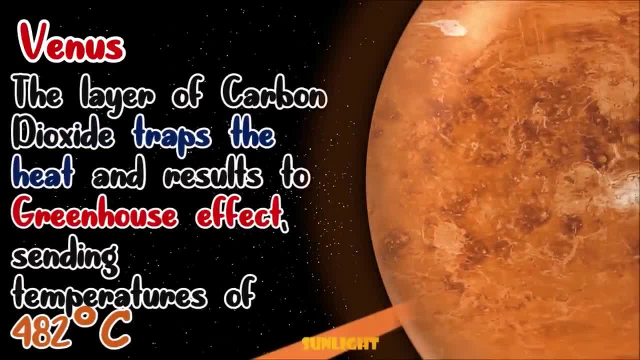 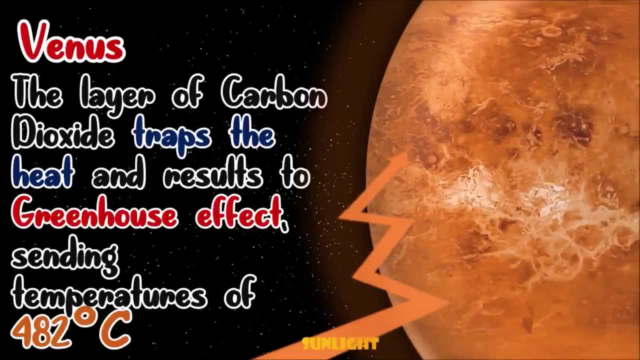 Venus is known as the hottest planet because of its very thick atmosphere made up of carbon dioxide. The layer of carbon dioxide drops heat and result to greenhouse gas. The viewer will feel that Venus is an electron of water Sun, junto with Saturn. chili is classified as an seulement잖아요 détectativo. 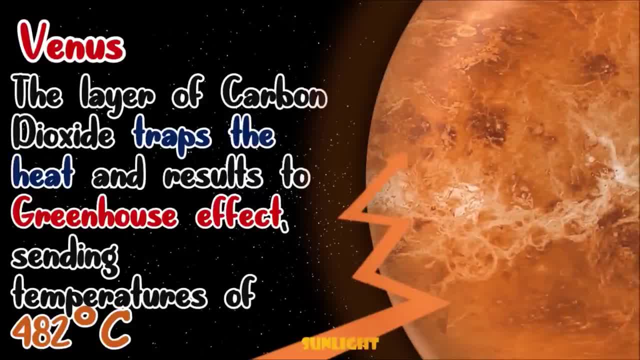 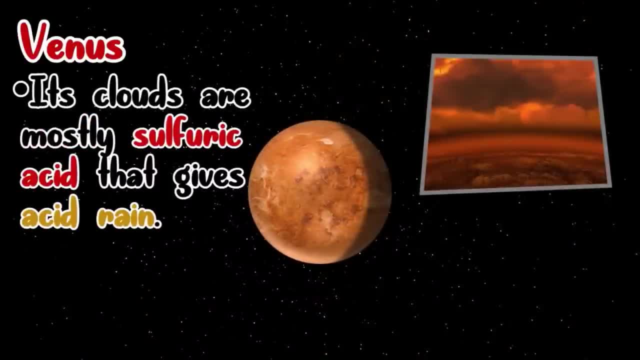 as it has a solar peak and reaches its maximum heat of 17.5°C. As a scientist from UK, he had suggested that Venus should beỉado of 64 Mondays. It is virtually impossible to Xn handy to the EU to determine the едwood and 3D. 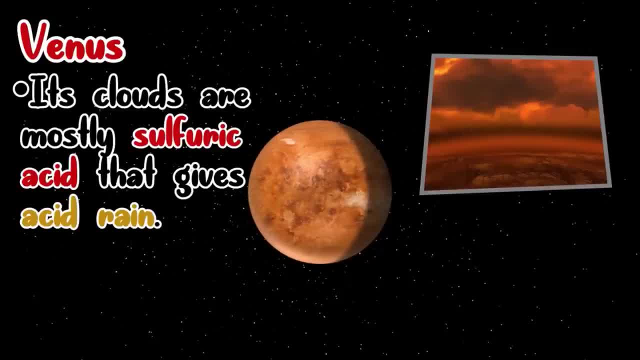 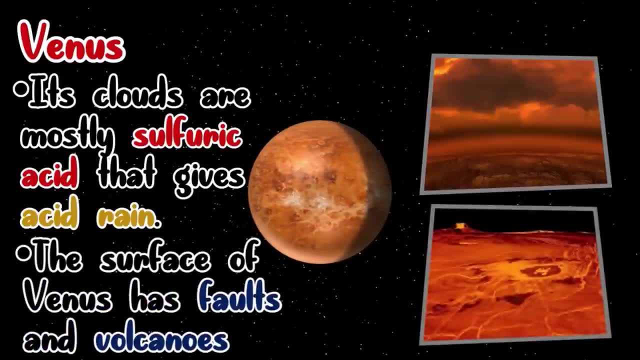 Labor flow in the other planets 🤩. They have been studied for decades but never revealed it, Since it has been lukewarm in a period of far enough time and under the enjoyable floating düsturm did they showFO govern soreness? 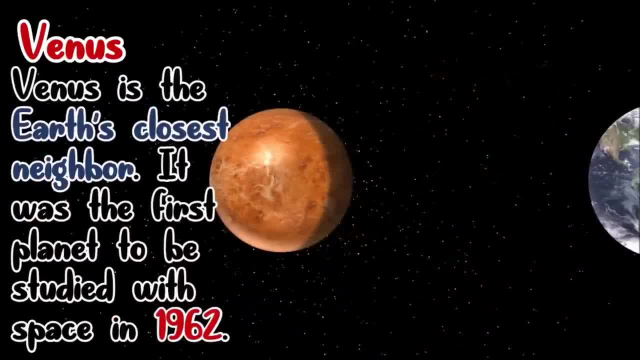 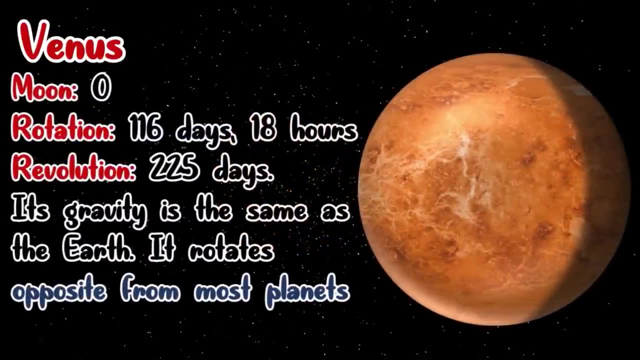 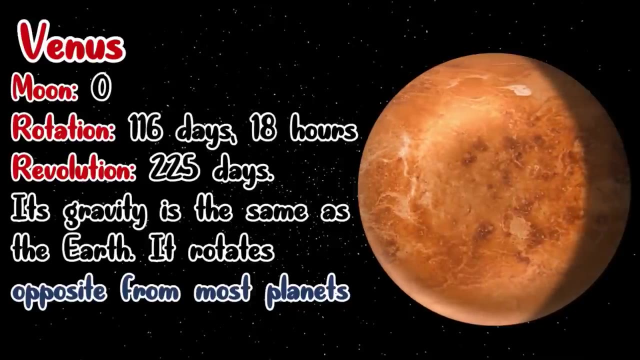 They also differ from the other planets: high and mid weather. here I wrote that Venus is the major coloured planet in the atmosphere and not the sun is the earth's closest neighbor. it was the first planet to be studied with space in 1962. venus has no moons and the gravity is as strong as the earth. a rotation of venus requires 116 days. 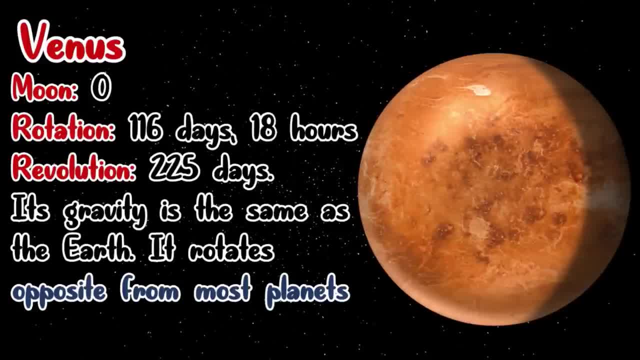 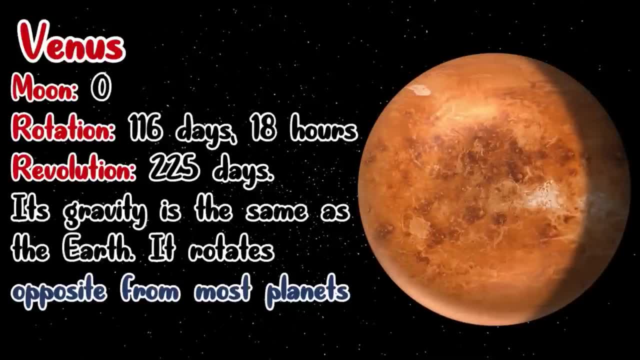 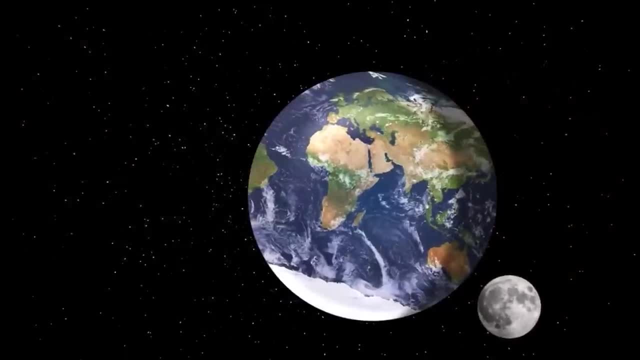 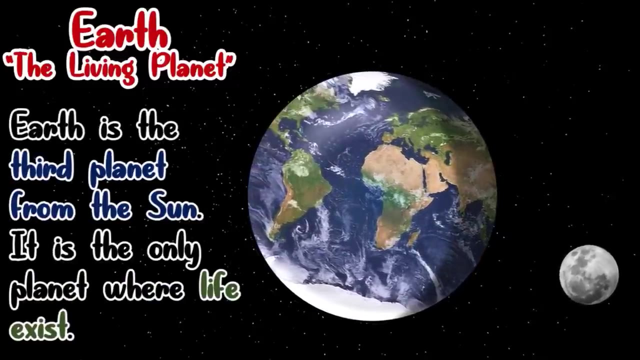 and 18 hours. however, its revolution requires 225 days. venus rotation is very slow that it only rotates two times in one year. the earth, earth, is known as the living planet. earth is the third planet from the sun. it is the only living planet where life exists. 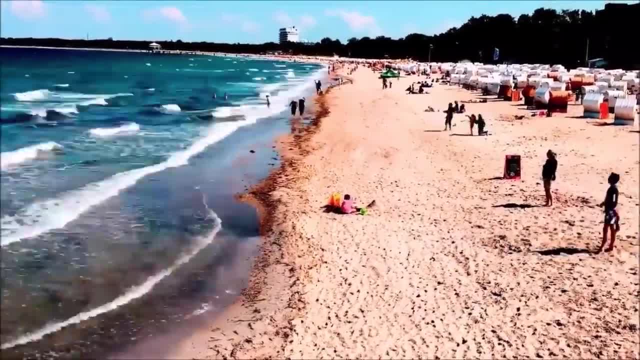 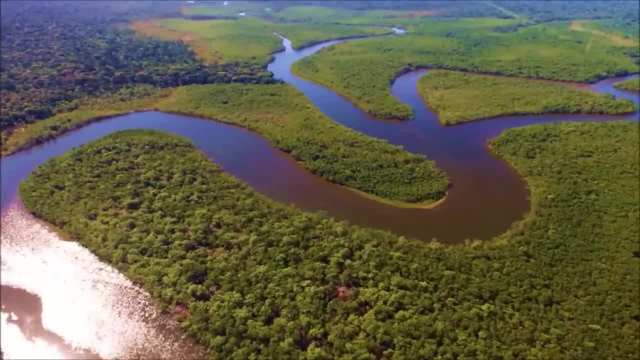 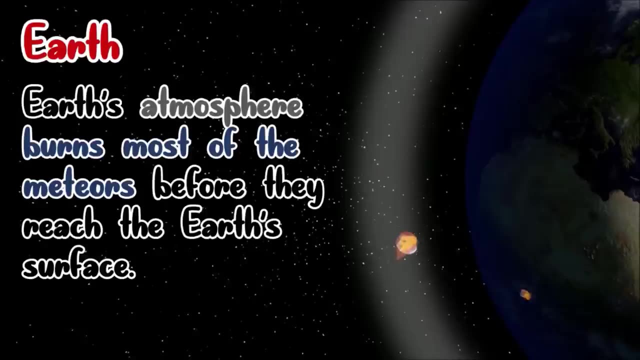 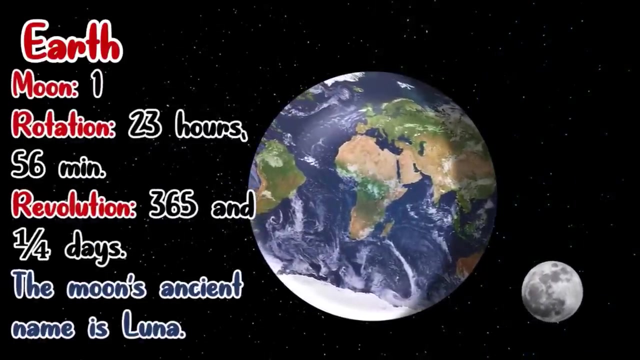 earth is rich in liquid water that supports life. it has atmosphere that supports and protects life. earth's atmosphere burns most of the meteors before they reach the earth's surface. the earth has one large moon. earth's rotation requires 23 hours and 56 minutes. 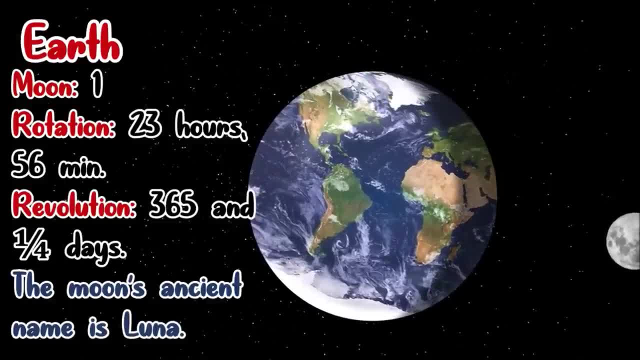 and a one-day rotation of 23 hours and 56 minutes. and a one-day rotation of 23 hours and 56 minutes and a one-day rotation of 23 hours and 56 minutes. one complete revolution of the earth takes 365 and one-fourth days. 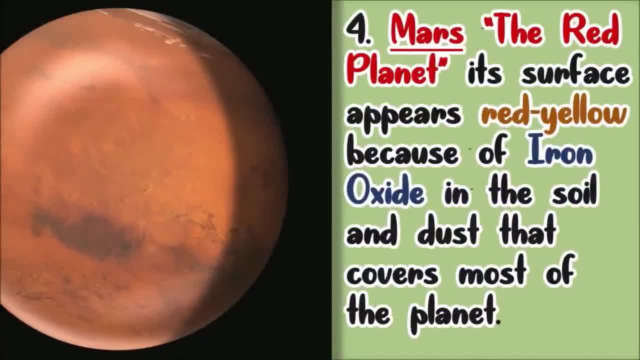 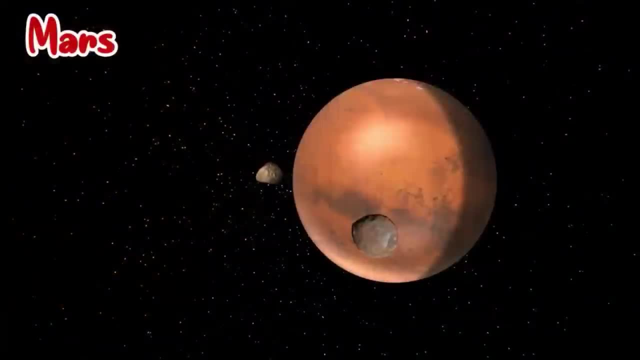 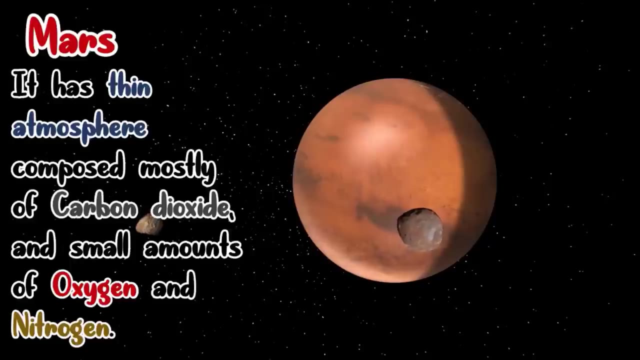 mars. mars is known as the red planet. its surface appears red, yellow because of iron oxide in the soil and dust that covers most of the planet. the red planet appears red and the earth is full of rise from the water. mars has a thin atmosphere composed mostly of carbon dioxide, small amounts of oxygen and nitrogen. 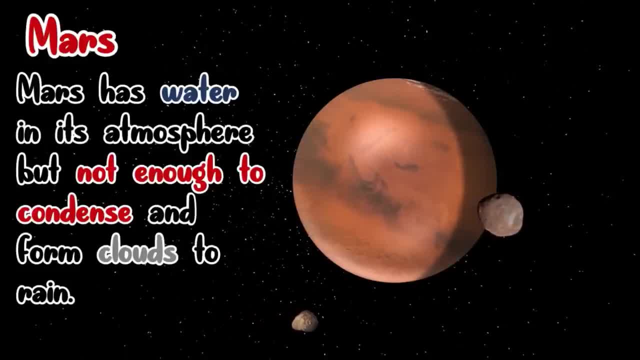 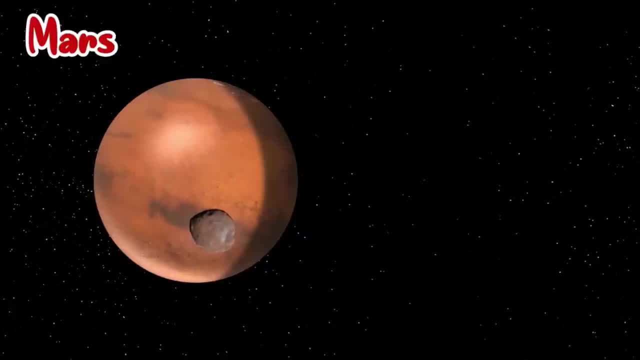 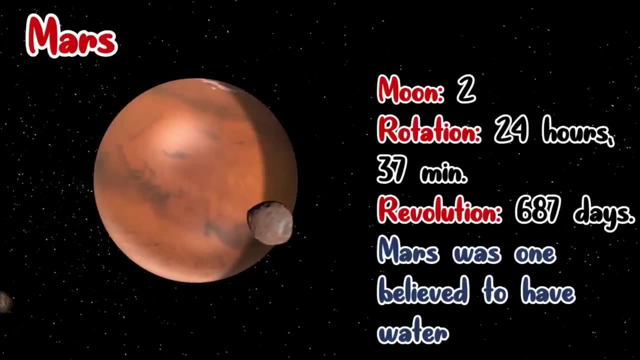 mars has water in its atmosphere, but not enough to condense and form clouds. the red planet is also known as the moon's head. days on mars are almost the same because the red planet is known as the sun's head same on Earth. a Mars rotation requires 24 hours and 37 minutes while it 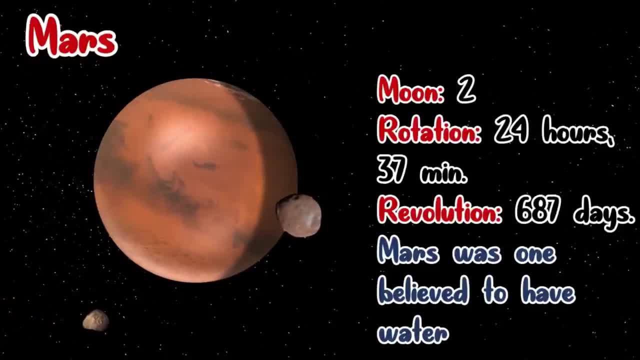 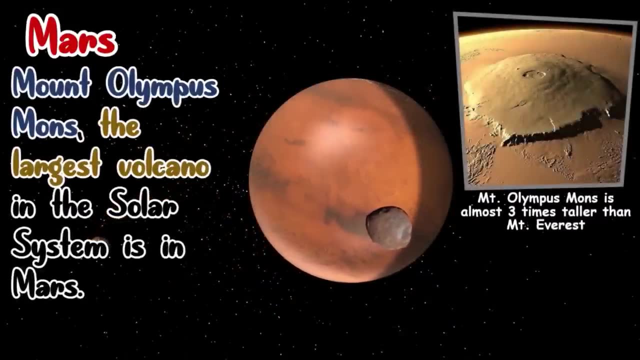 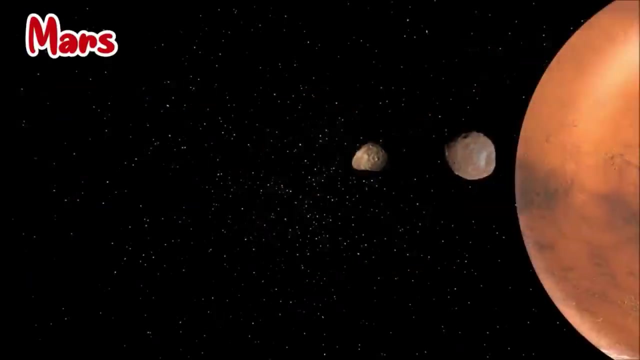 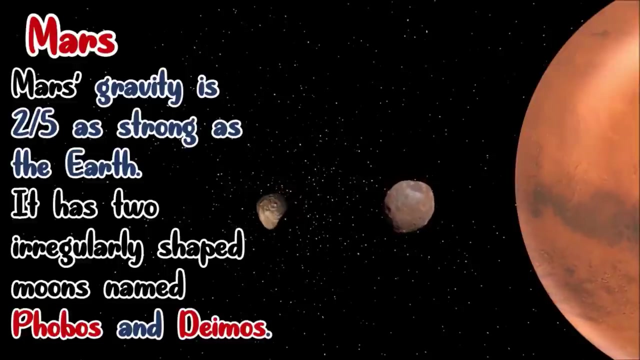 requires 687 days to complete a one revolution. Mars was once believed to have water. the largest volcano in the solar system is also found in Mars. it is called Mount Olympus month. Mars gravity is two-fifths as strong as the earth. Mars has two irregularly shaped 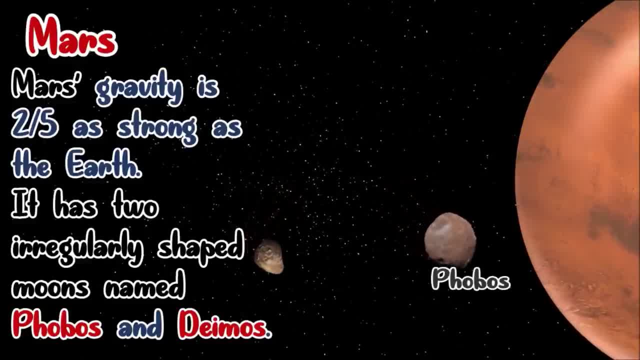 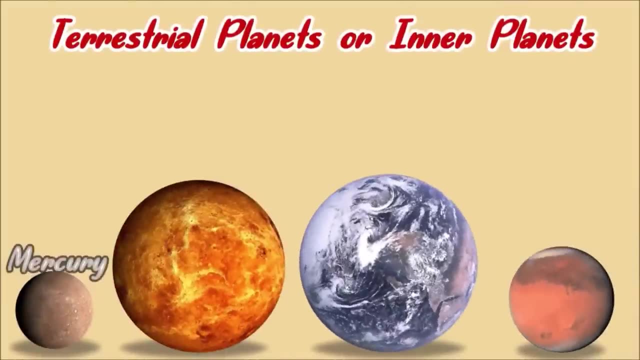 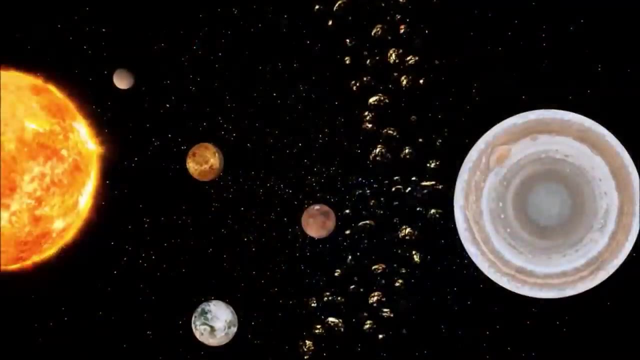 moons, it is called Phobos and Dimas. Mercury, Venus, Earth and Mars are two-fifths as strong as the earth House are called terrestrial planets because they have ruckus surfaces and metal course. now, what are these things between Mars and Jupiter? these are group. 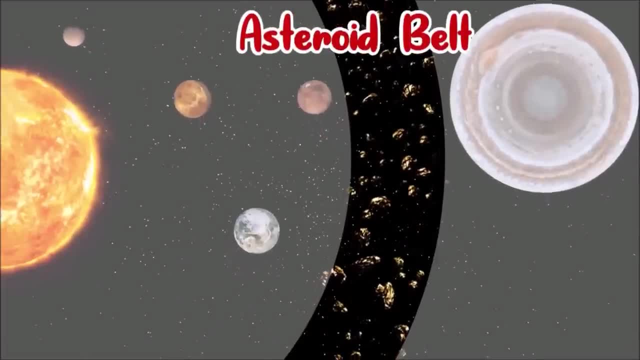 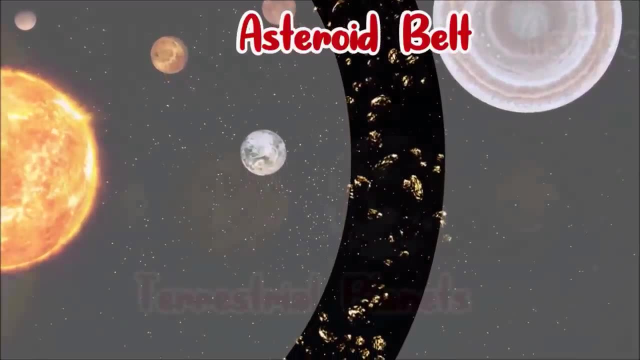 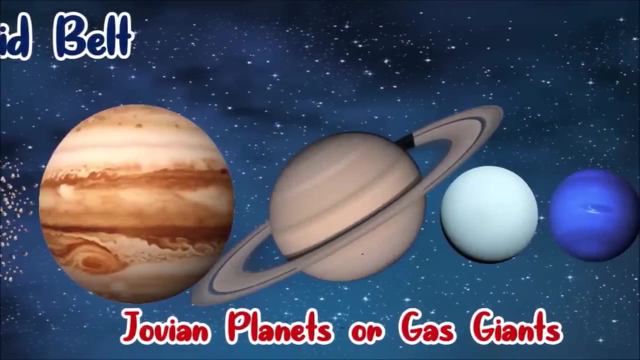 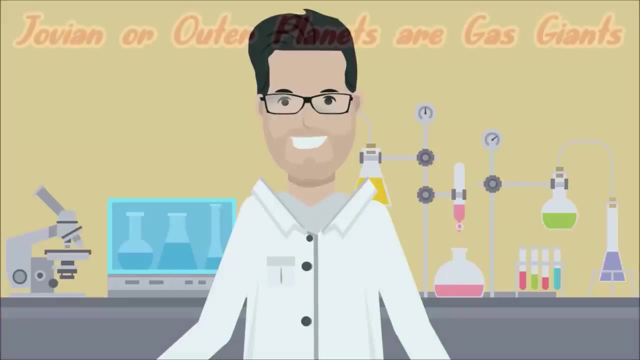 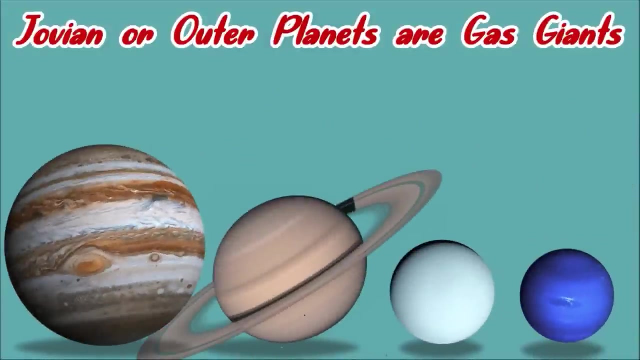 of asteroid. this is called asteroid belt. an asteroid belt is found between the orbit of Mars and Jupiter. the asteroid belt separates the terrestrial planets and the Jupiter, Jovian or gas giants. let's talk about the outer planets. these planets are known as gas giants. these are Jupiter, Saturn, Uranus and Neptune. this is 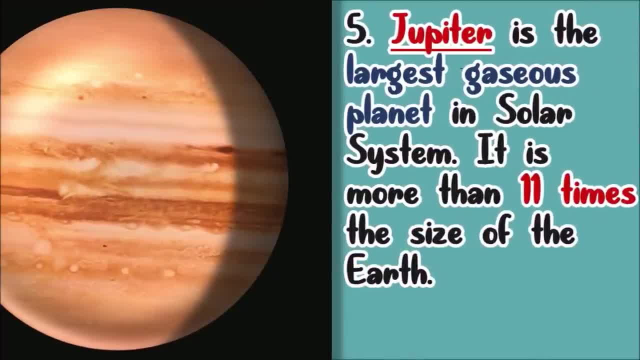 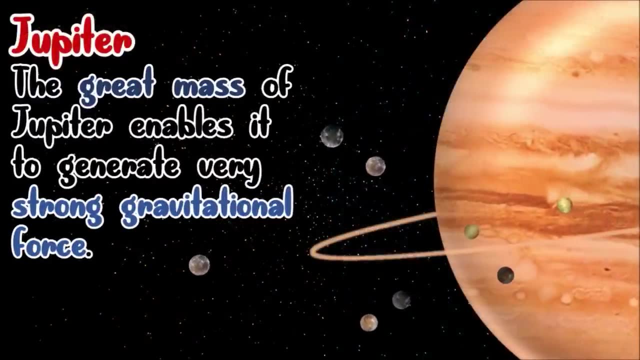 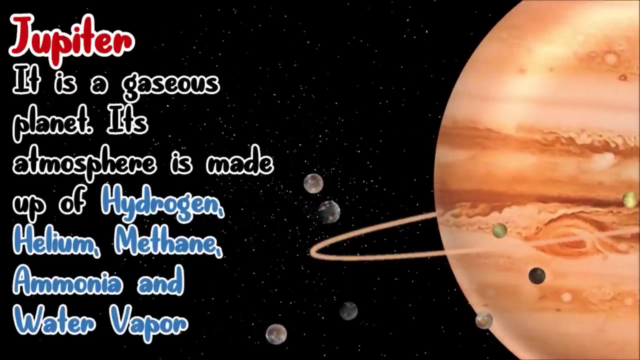 Jupiter. Jupiter is the largest gaseous planet in our solar system. it is more than 11 times the size of Earth. the great mass of Jupiter enables it to generate very strong gravitational force. Jupiter is a gaseous planet. its atmosphere is made up of hydrogen. 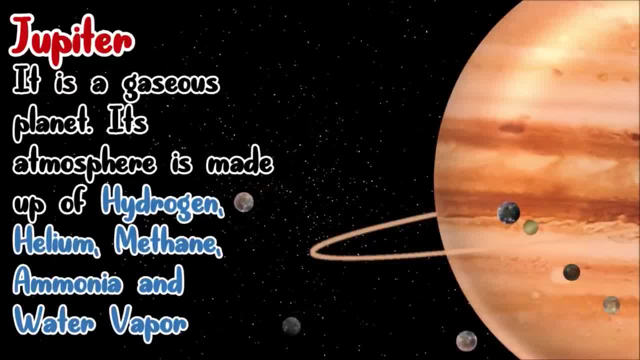 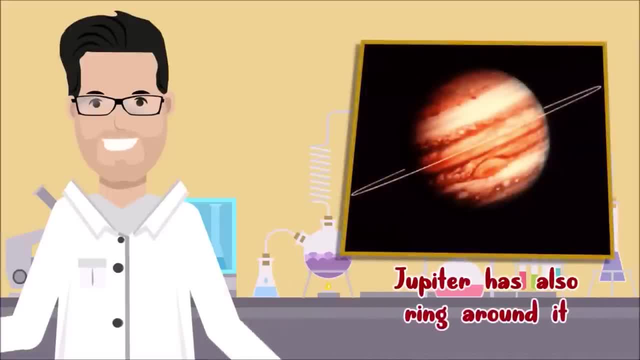 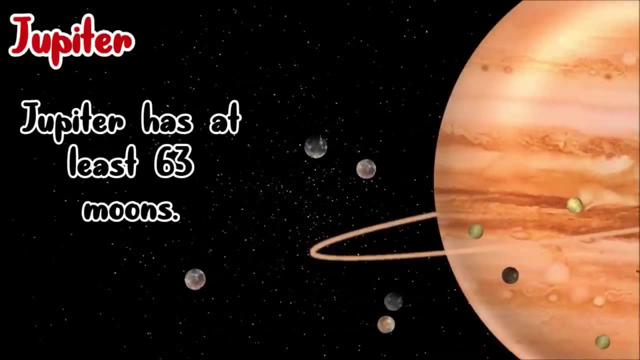 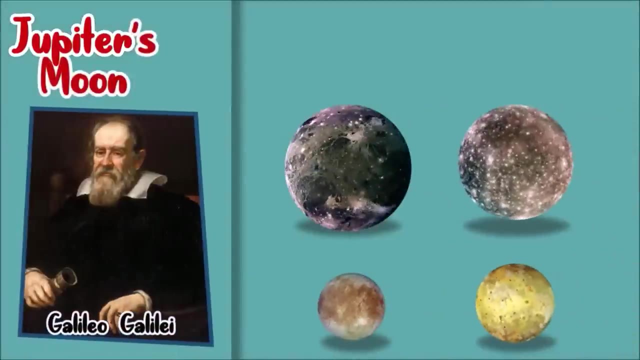 helium, methane, ammonia and water vapor. did you know that Jupiter has a very small, faint dust rings around it? Jupiter has at least 63 moons. four moons were first observed by Galileo Galilei and was named Galilean moons. some of the moons of Jupiter are Ganymede. 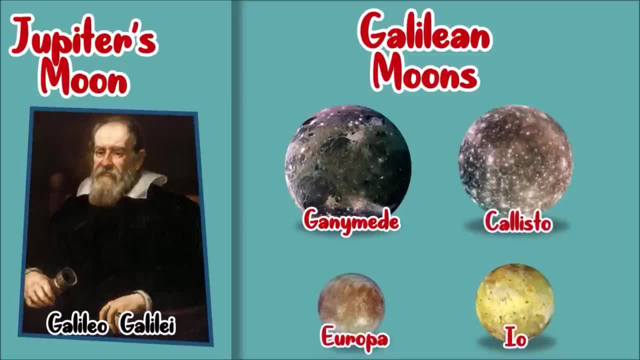 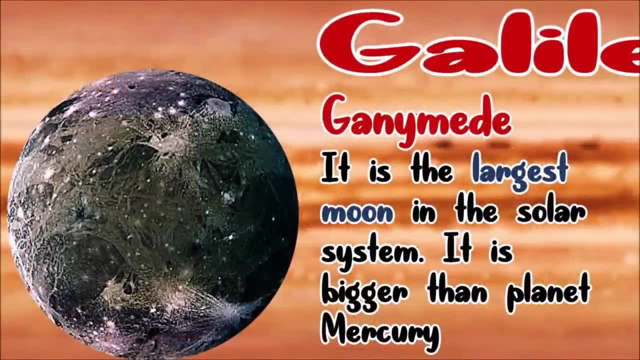 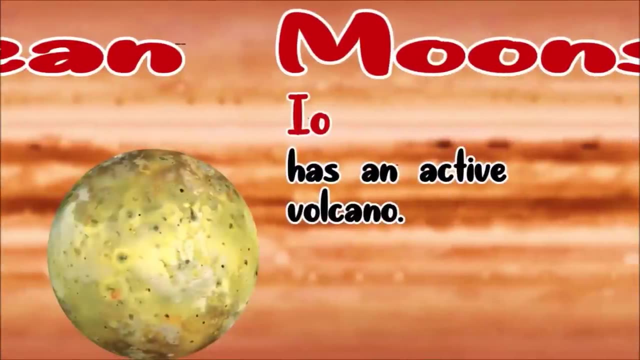 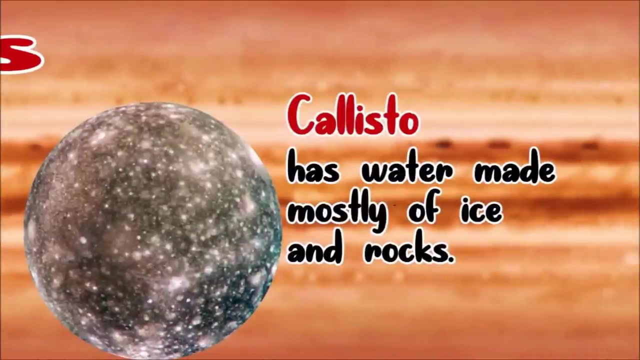 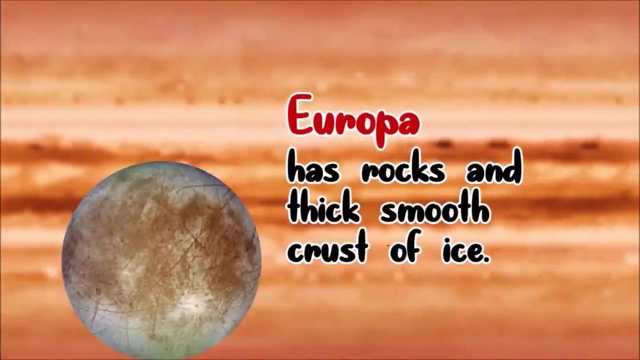 Callisto, Europa and Io. Ganymede is the largest moon in the solar system. it is actually bigger than Mercury moon. Io has an active volcano, while Callisto has water made mostly of rocks and ice. her background and move ever since Jupiter overflowed with electrostatic. 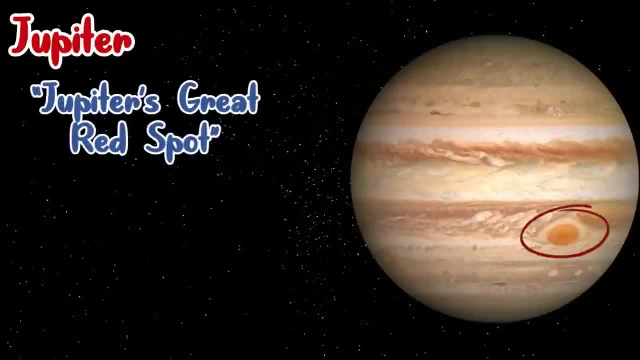 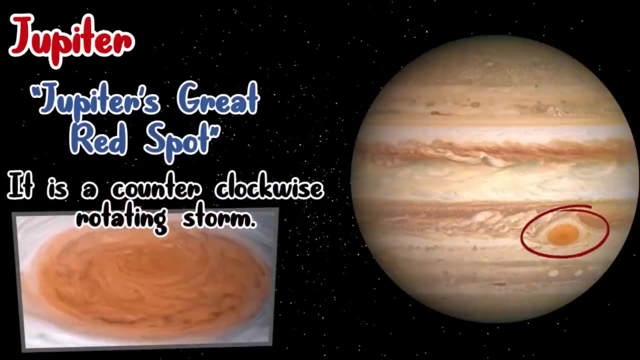 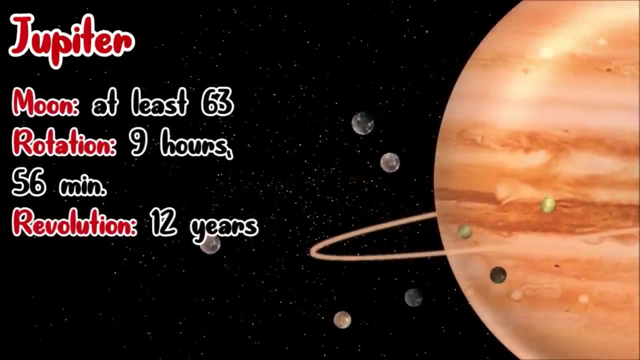 both of these rotations had an impact on our bizarre religious assembles and bellwether retardation. here we see the parasitic Jackie. I can't tell you which no Policy research talk is going on this morning. the present participants have said that if Jupiter was in a low altitude and or 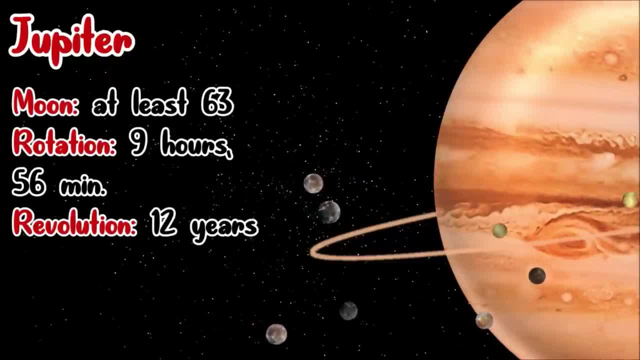 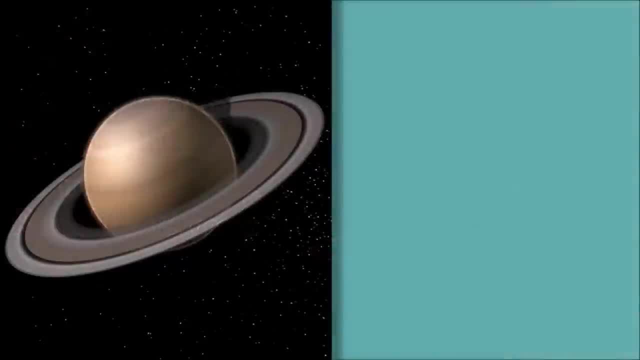 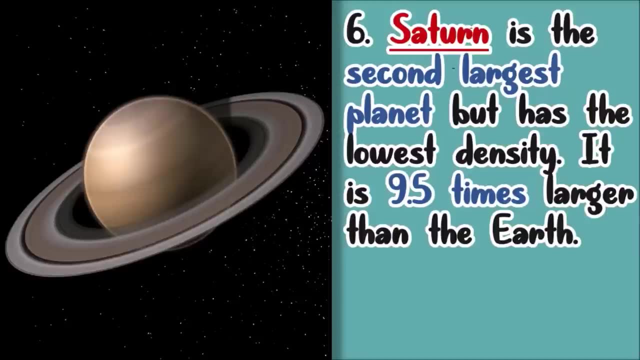 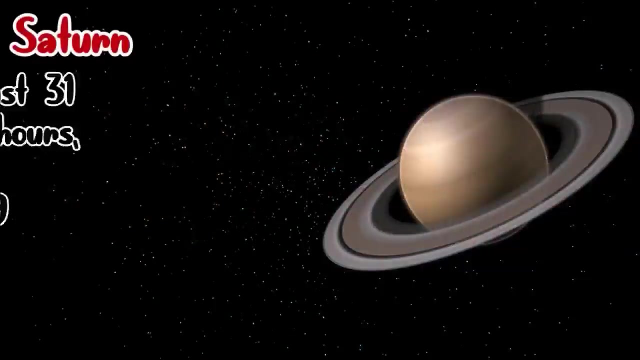 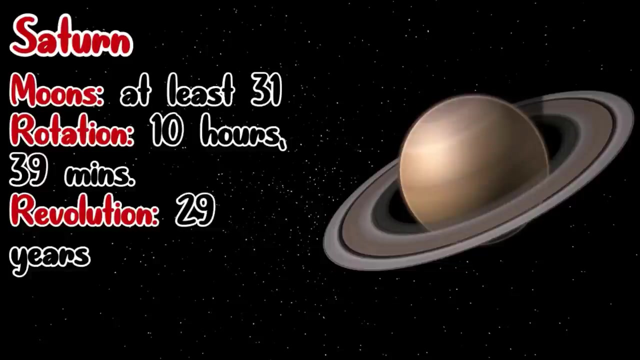 greater into the Gத region with people and further которых fulleka hers 分 ingern 噴 sun, saturn. saturn is the second largest planet, but has the lowest density. it is nine and a half times larger than the earth. its rotation requires 10 hours and 39 minutes. it requires 29 years to complete a revolution around. 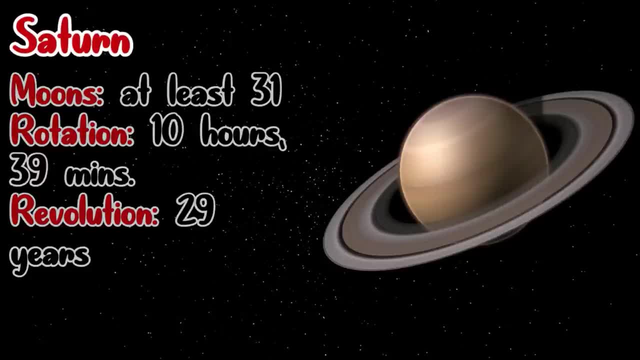 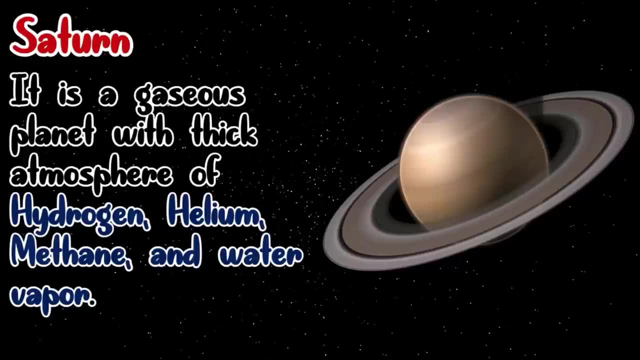 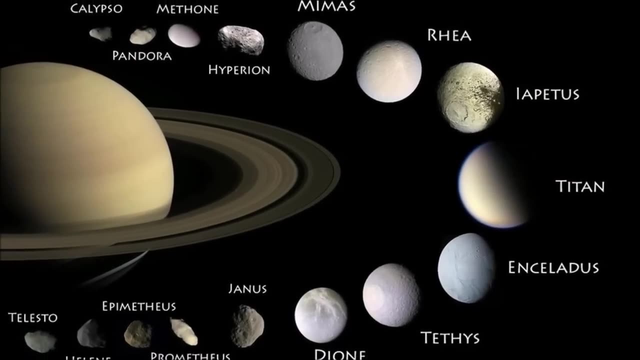 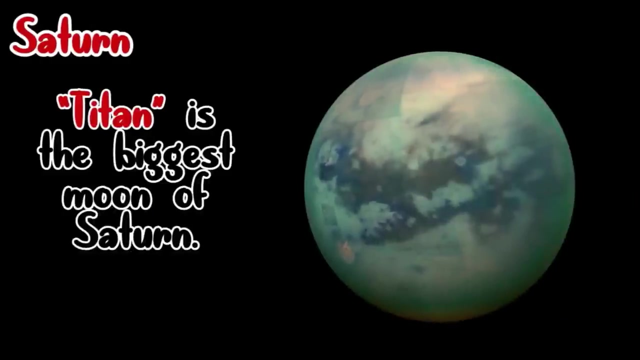 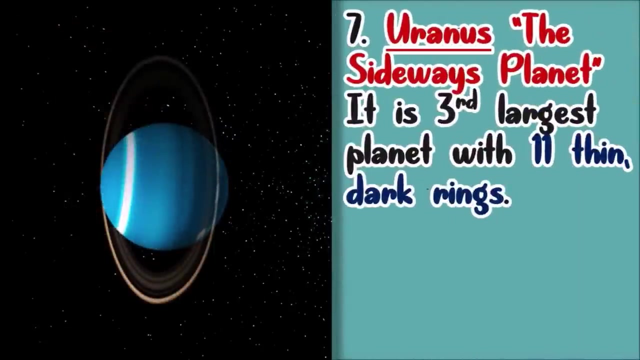 the sun. saturn is a gaseous planet. it has a thick atmosphere of hydrogen, helium, methane and some water vapor. saturn has at least 31 moons and the largest moon of saturn is called titan uranus. it is also called the sideways planet. uranus is the third largest planet, with a system of 11 thin dark rings. 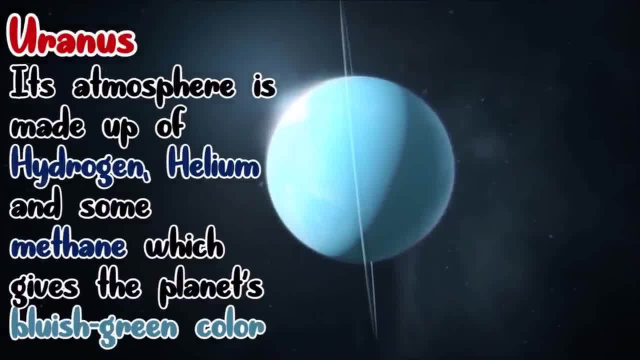 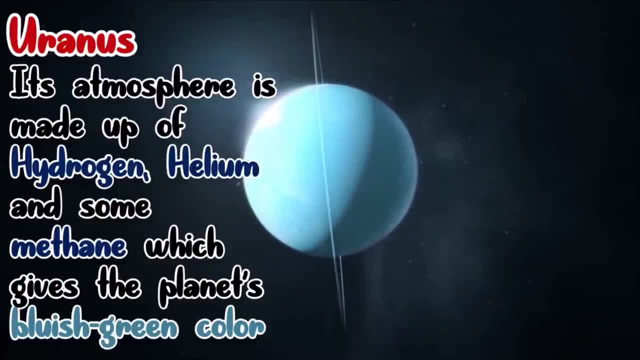 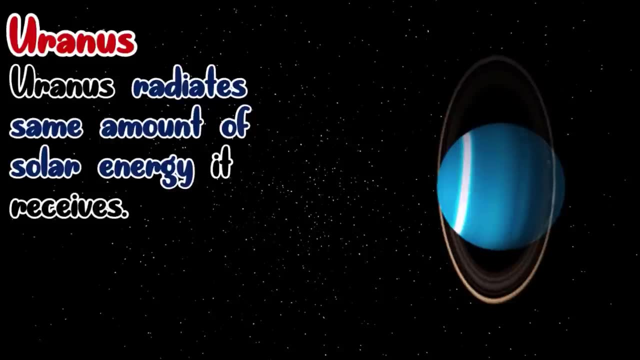 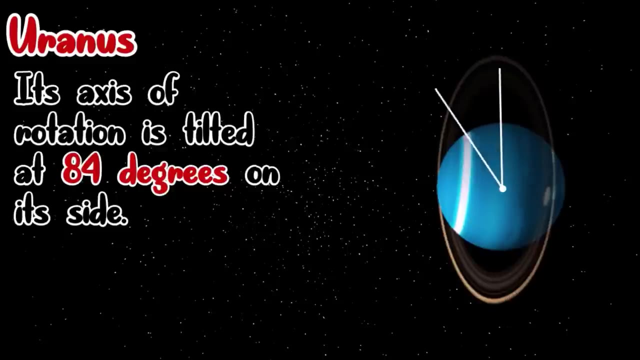 its atmosphere is made up of hydrogen helium and some methane, which gives the planet a bluish green color. uranus radiates the same amount of solar energy it receives. uranus axis of rotation is tilted at 84 degrees on its side. the result is its north pole faces the sun. 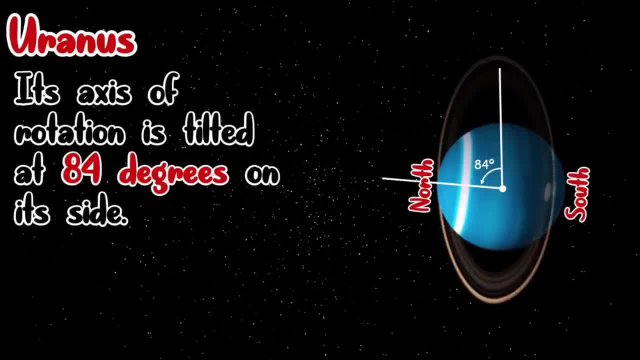 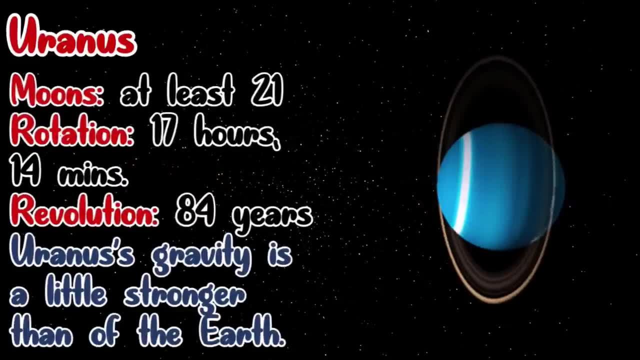 for one half of 84 years revolution. Uranus requires 17 hours and 14 minutes in every rotation, And to complete a revolution around the Sun, it requires 84 years. Uranus' gravity is a little stronger than of the Earth. It has at least 21 moons, The largest moon of 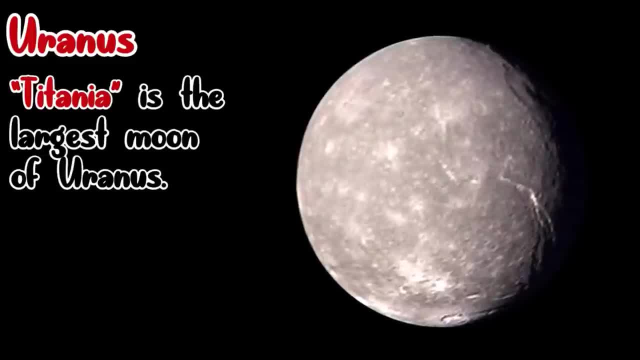 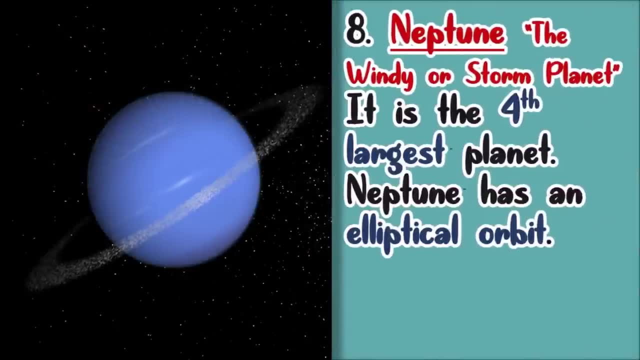 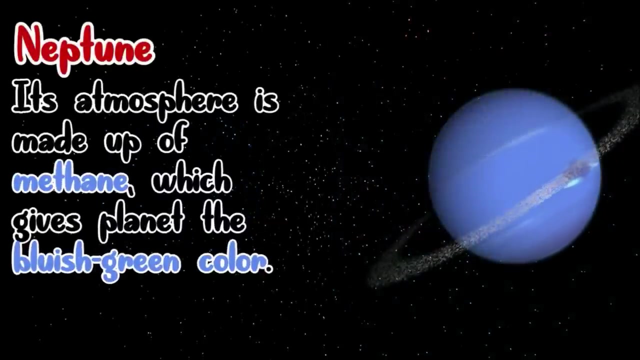 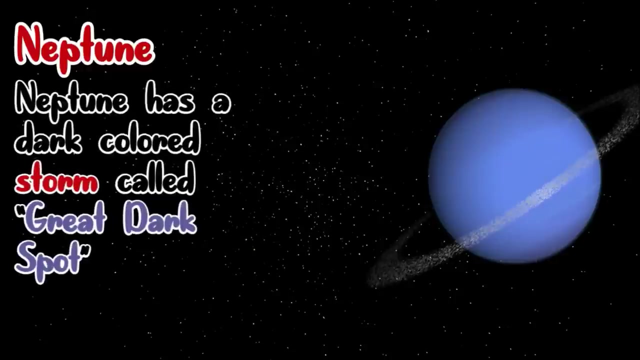 Uranus is called Titania Neptune. It is the windy planet, or also called as storm planet. Neptune is the fourth largest planet. Neptune has an elliptical orbit. Its atmosphere is made up of methane, which gives the bluish green color. Neptune has a dark-colored storm. It is called Great Dark Spot. 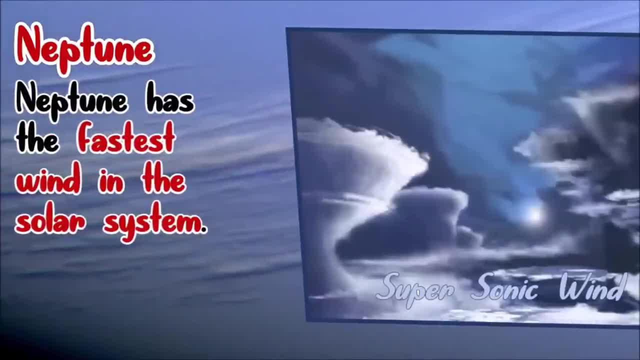 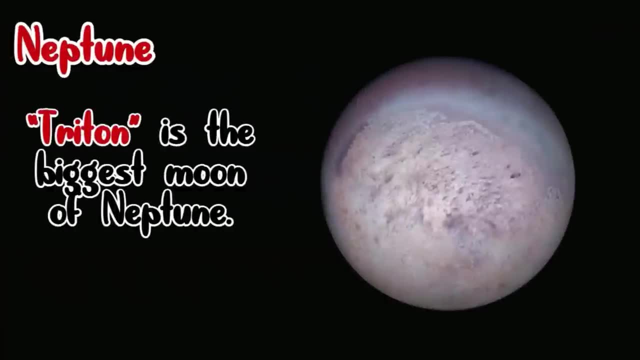 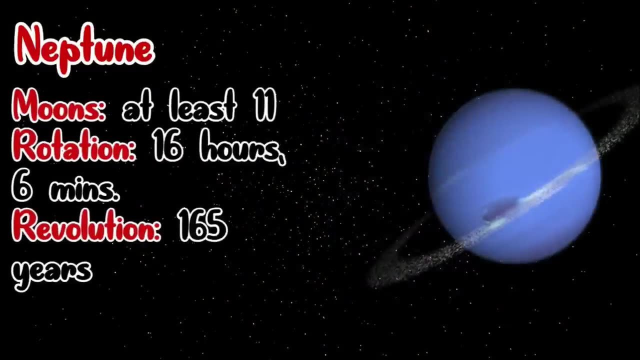 Neptune has the fastest winds in the solar system. It has at least 11 moons. The largest moon of Neptune is called Triton. Neptune's rotation requires 16 hours and 6 minutes, And to complete a one revolution around the Sun, it requires 165 years. 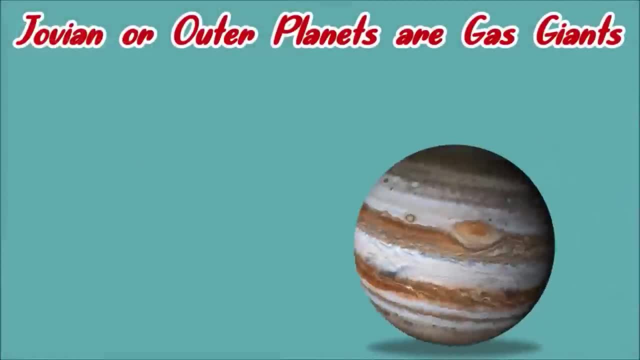 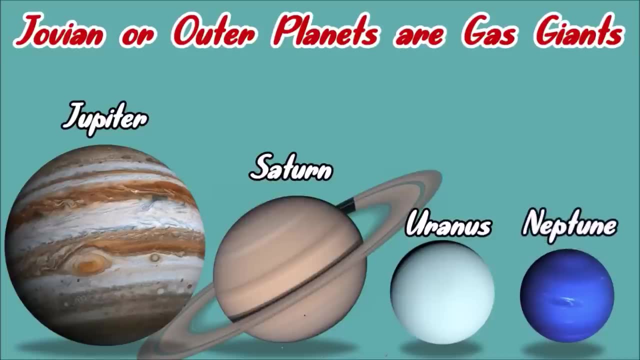 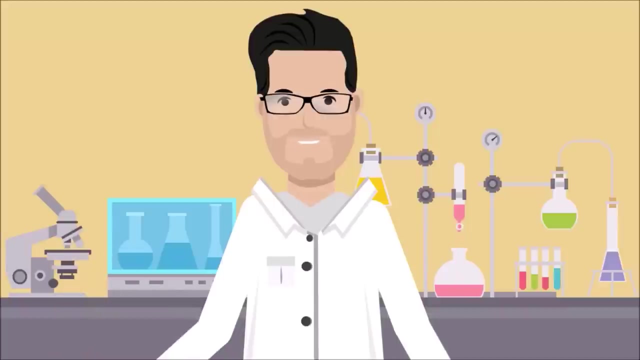 And these are the Jovian planets or the four gas giants. Can you enumerate the planets of the solar system? by which is the closest and the farthest planet from the Sun? Let's say it one by one. Let's say it one by one. 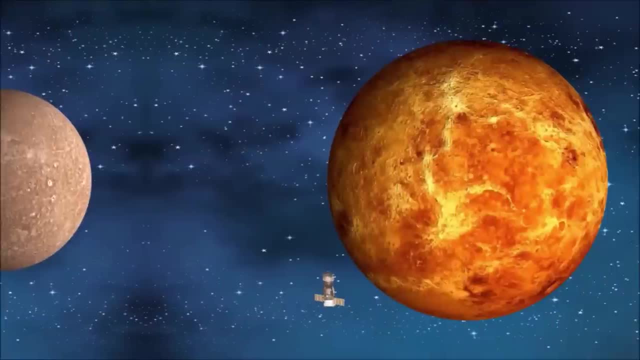 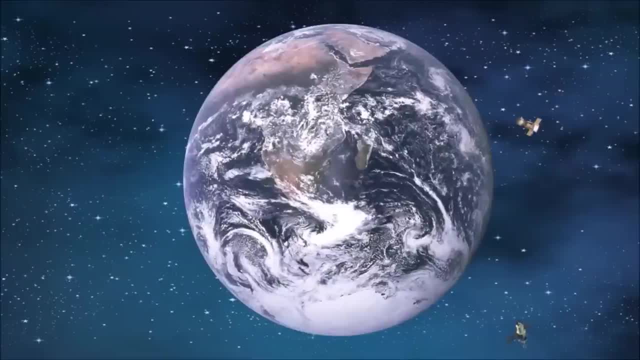 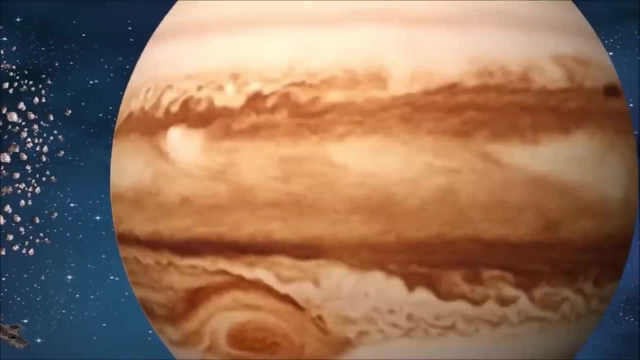 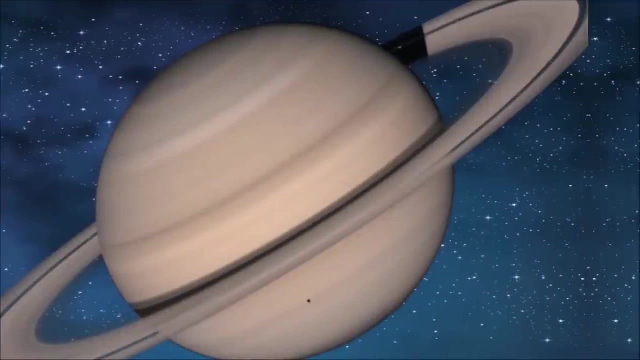 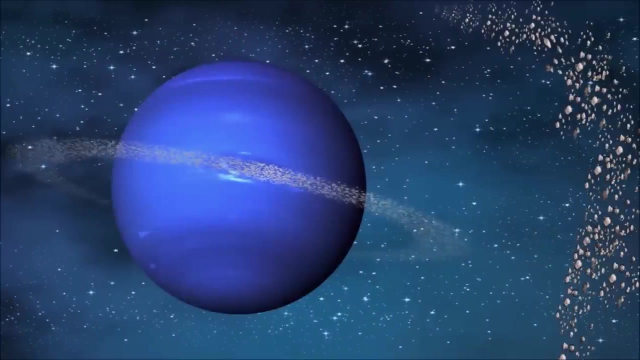 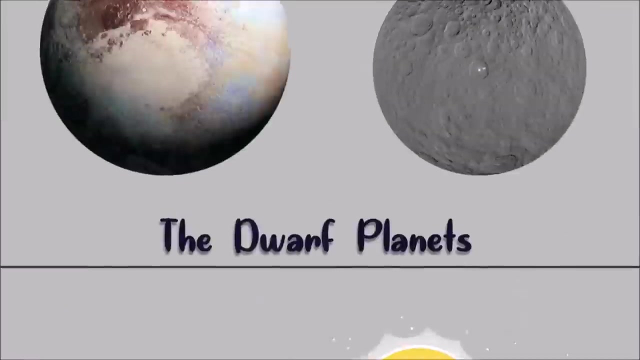 Let's say it one by one: Watch this When, When, If not now? Yes, Yeah, Wow, That feeling is like Rogan. Yeah, You have to learn HOW to use an arm. now let's talk about the dwarf planets. some of the example of dwarf planets are: 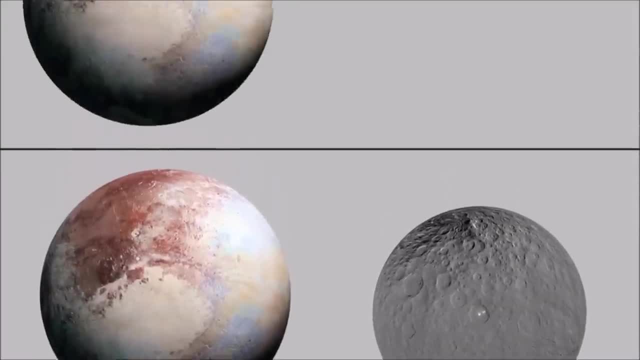 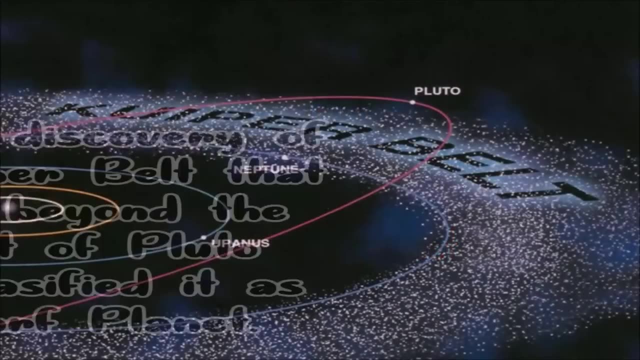 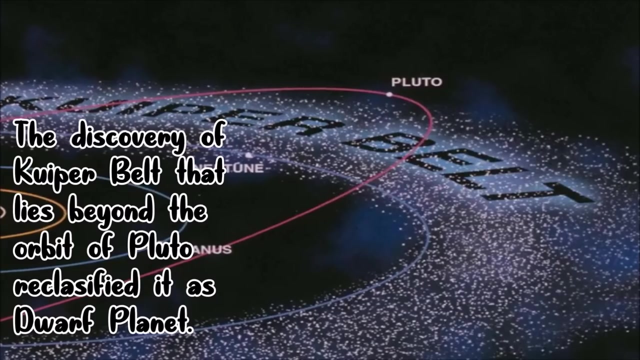 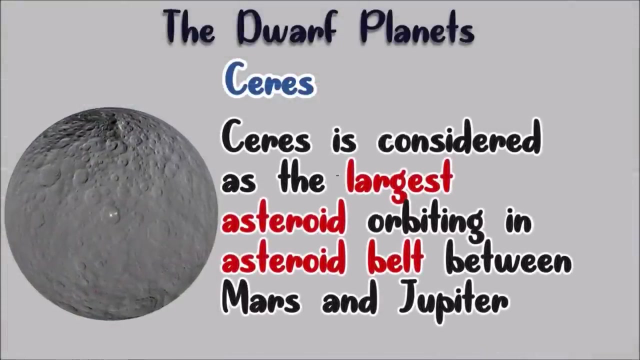 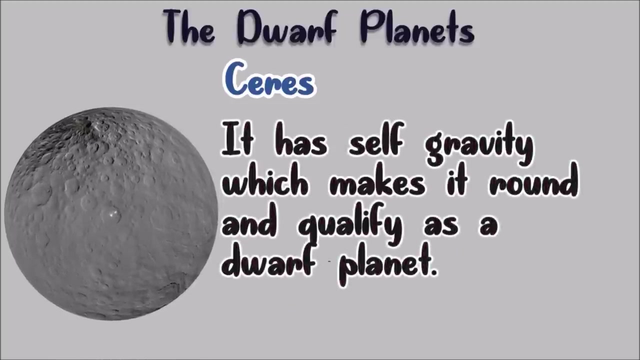 Pluto and Ceres. Pluto was considered the ninth planet until 2006. the discovery of Cooper belt, that lies beyond the orbit of Pluto, reclassified it into a member of dwarf planet Ceres. Ceres is considered as the largest asteroid orbiting between Mars and Jupiter. it has self gravity, which makes it round and qualify as dwarf planet. 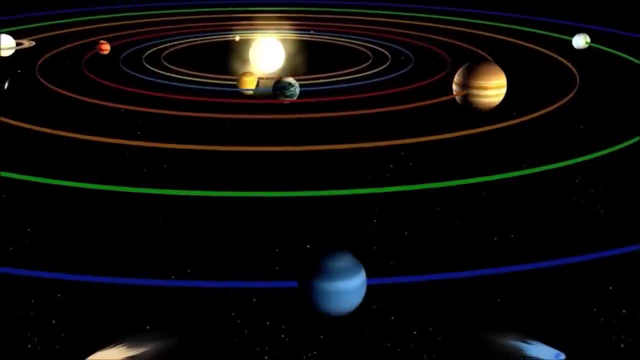 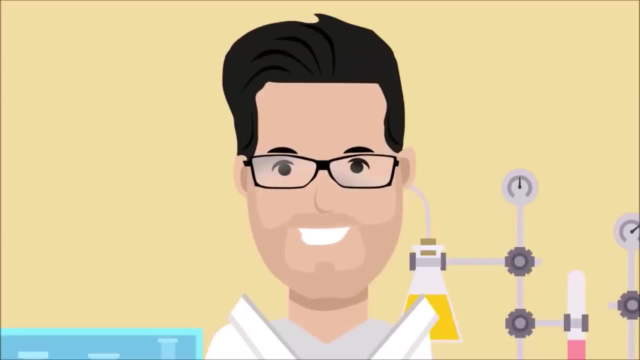 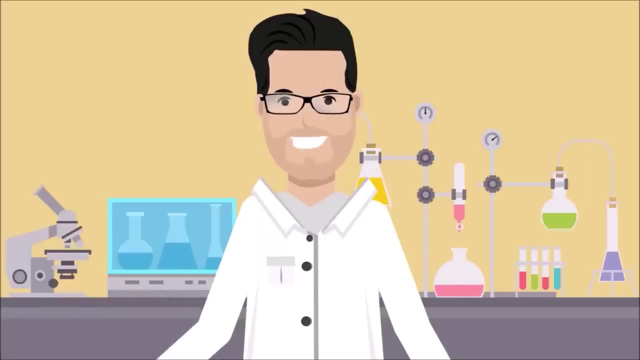 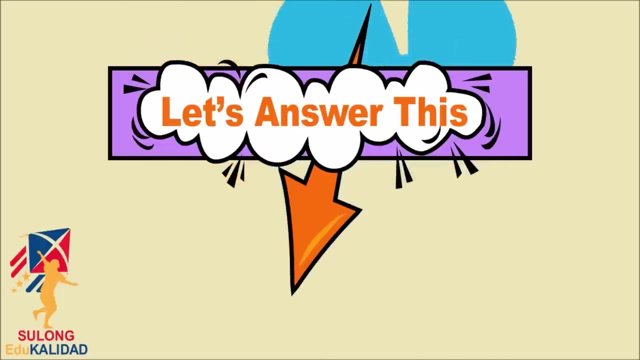 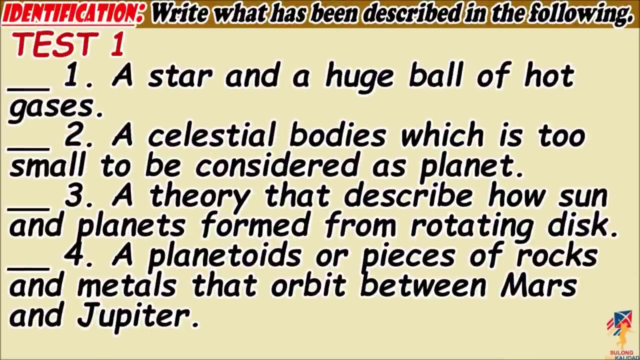 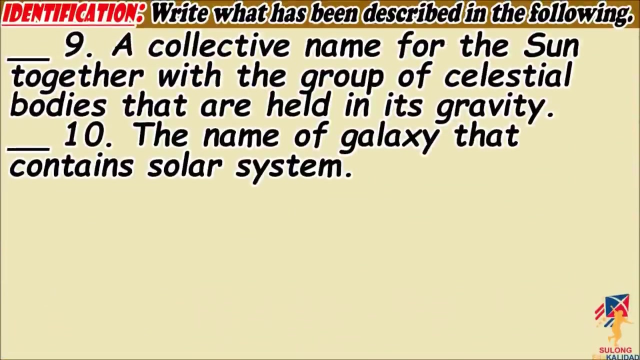 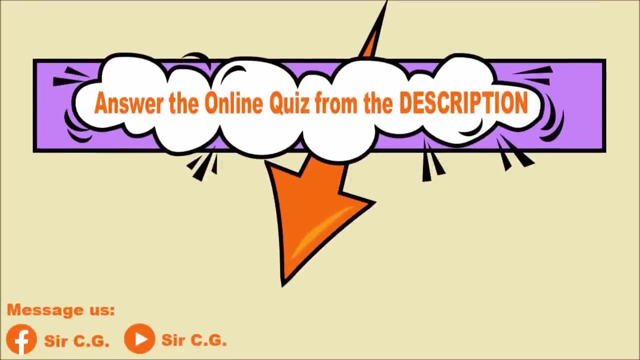 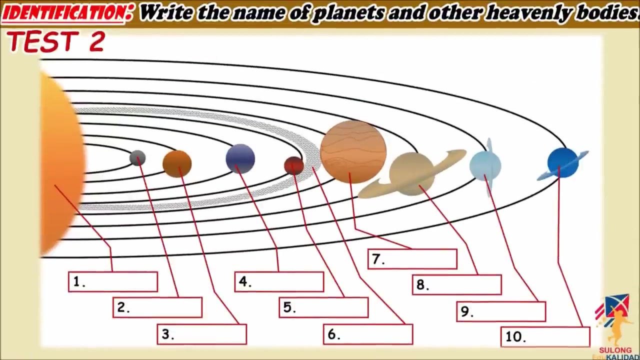 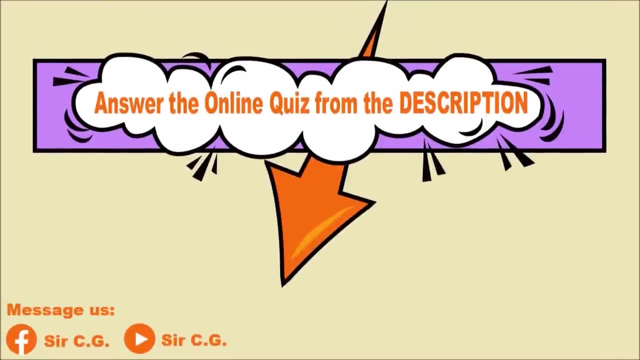 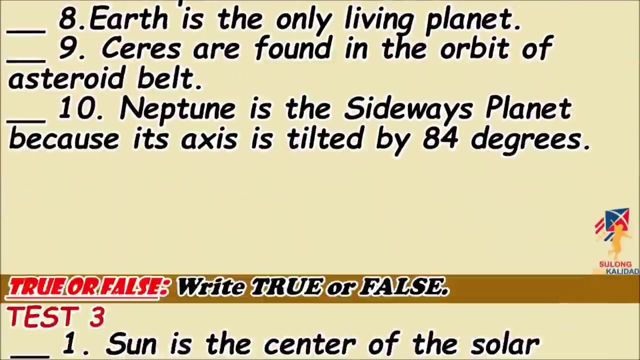 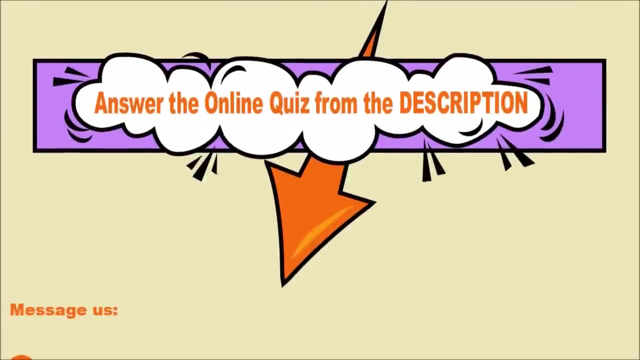 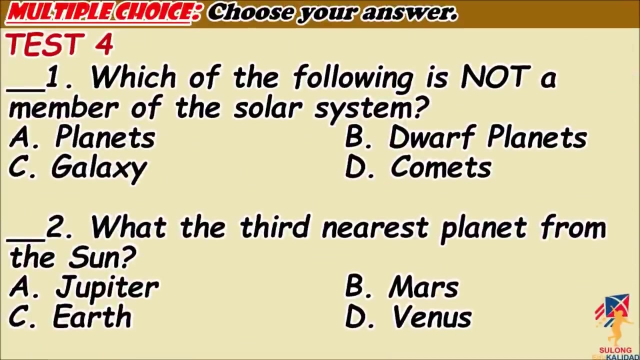 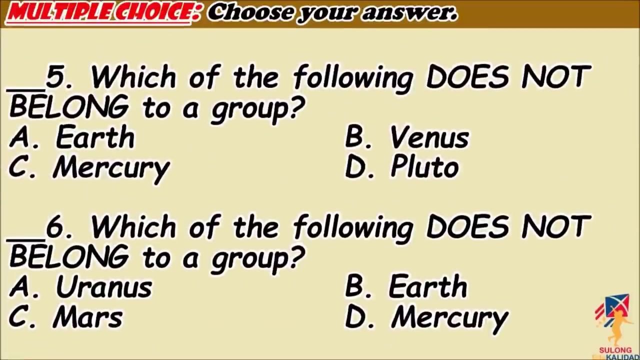 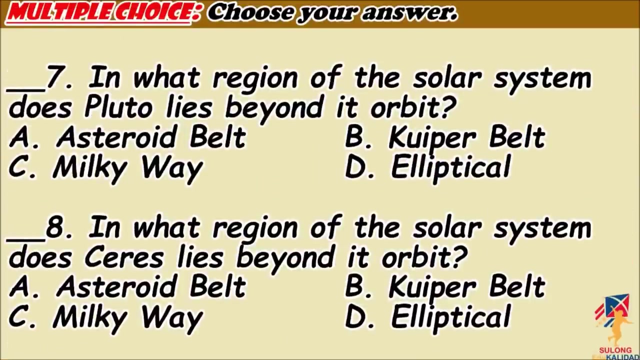 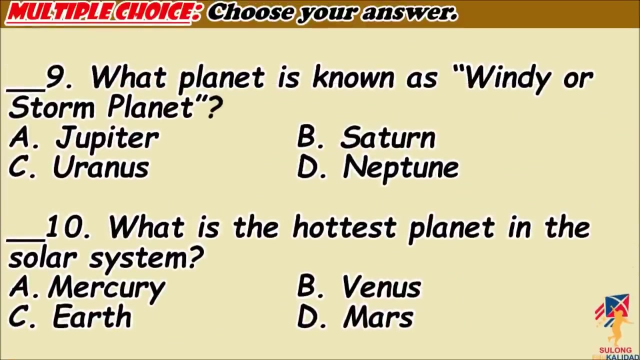 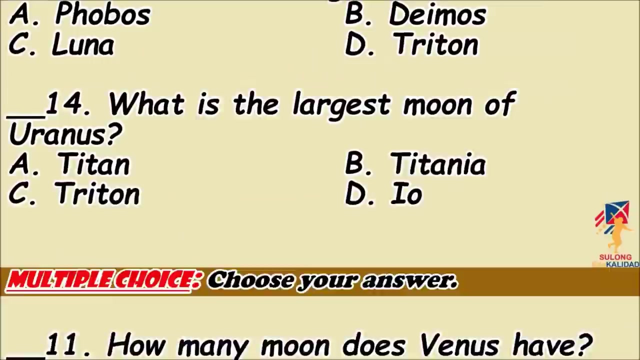 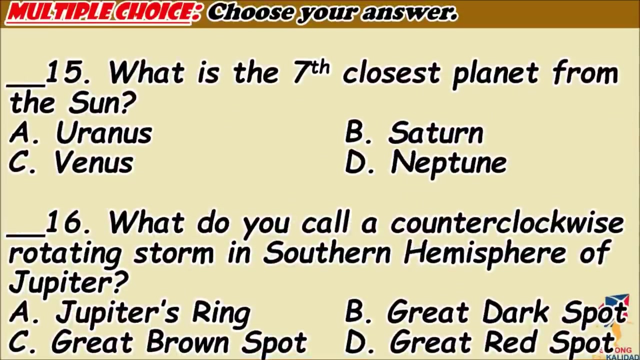 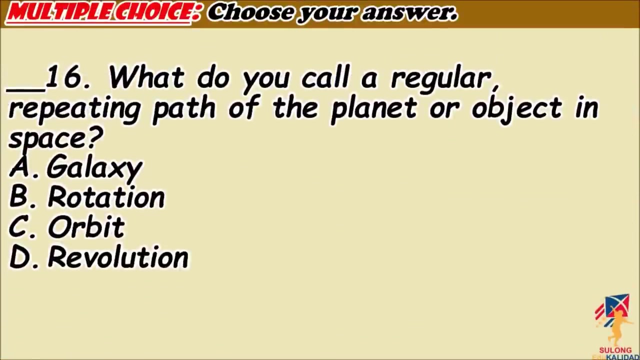 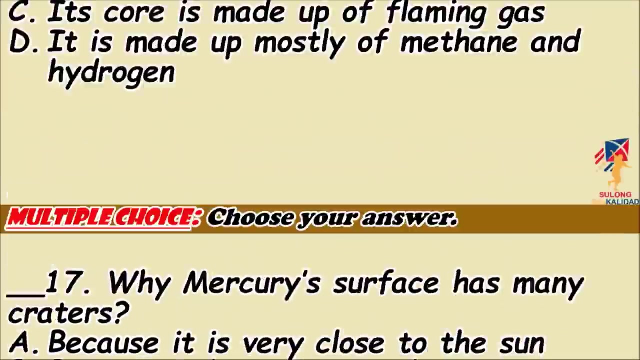 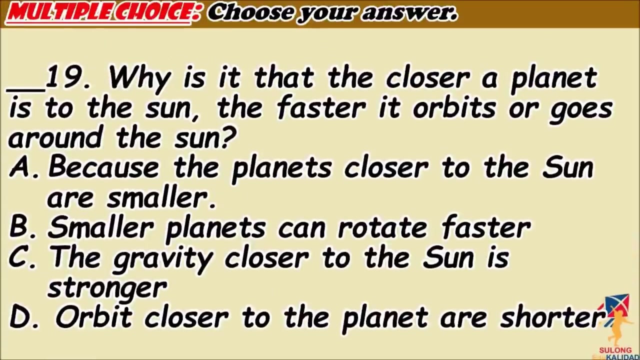 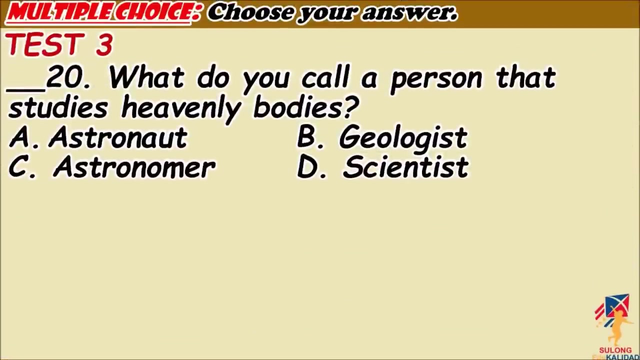 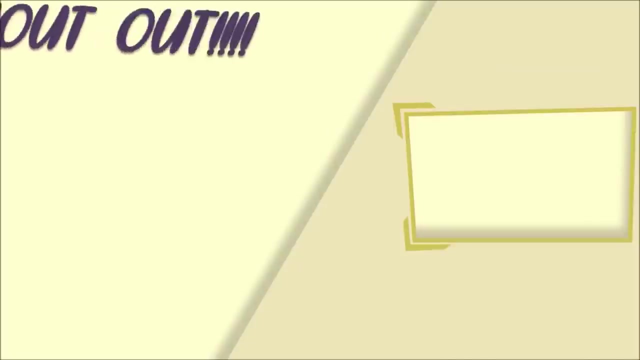 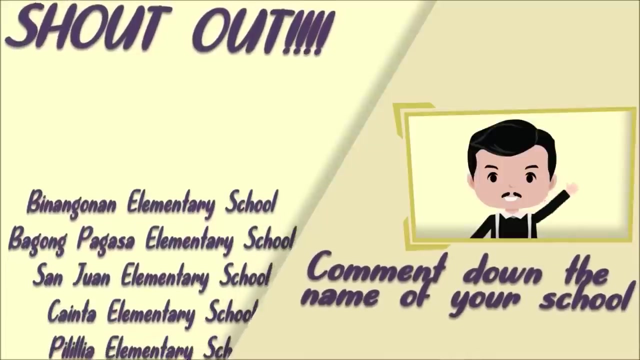 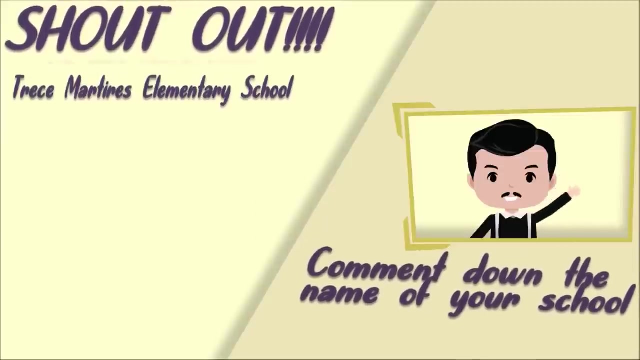